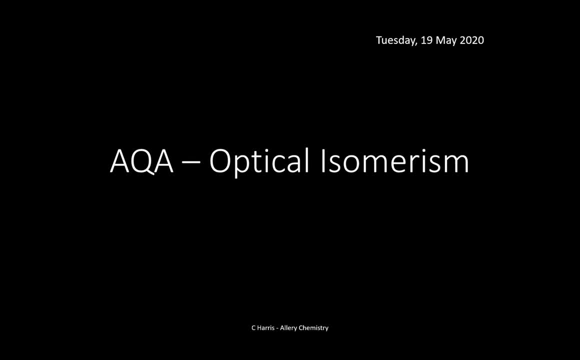 might find online the videos and documents that you might see. that may not be specific, You know they're just general information, which is fine, but this information you see on here is actually dedicated to AQA, so you don't have to worry about. is this going to be on the spec? is? 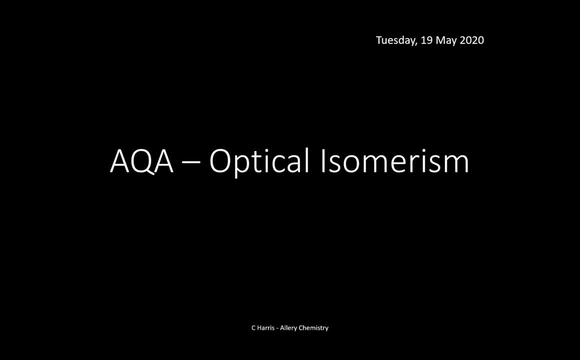 it not. Everything in here is for AQA, and likewise I've done a full series of AQA videos for year one and year two on Allery Chemistry YouTube channel. All I ask is that you hit the subscribe button, because they're all for free, so don't charge for them. 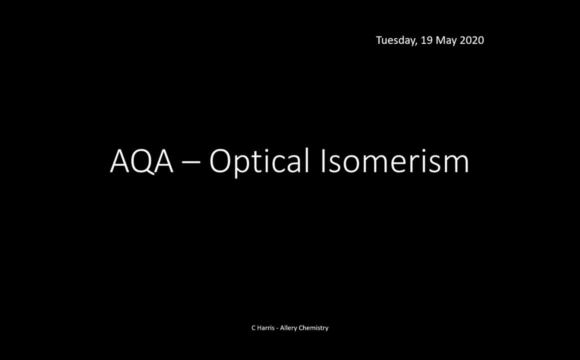 You hit the subscribe button and that'll be fantastic just to show you support. and as long as people keep subscribing and watching the videos, then I will keep making them Also on that channel. I suppose on that, on that point, there's also some. I do have some generic whiteboard videos as well. 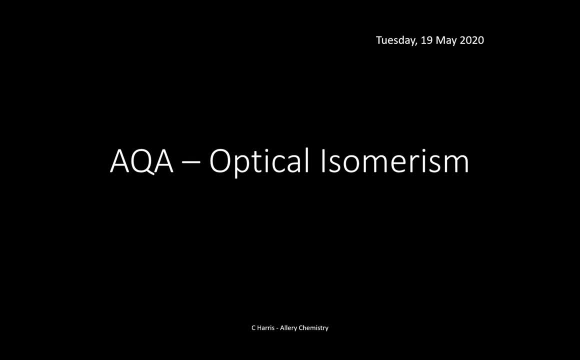 whiteboard tutorials where I go through specific areas of chemistry, and also I've got some some some past paper walkthroughs- and mine went blank there- some past paper walkthrough questions where it basically tries to improve the exam technique, But it's it's constantly adapting and changing and evolving, so you know to keep up to date then 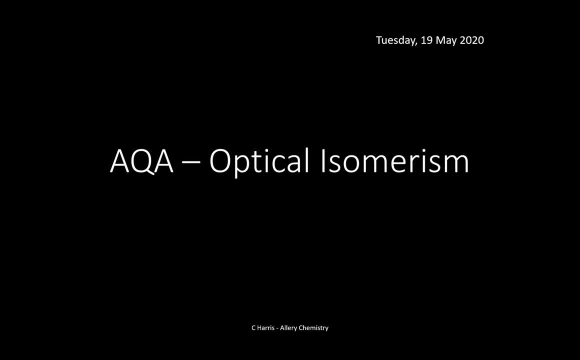 press the subscribe button. The video here is actually made from a PowerPoint presentation that I've made as part of a revision series of resources. They're available in the link. so if you click on the link in the description box, they're available there. They're good value for. 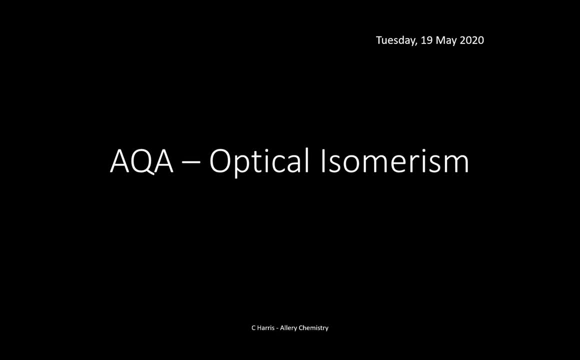 money. There's a full range from year one and year two, and you can use them on your smartphone or you can use them then, and I've known some people actually print off the slides as well and use them as revision notes. So feel free to you know to do that. click on the link. you'll be able to purchase. 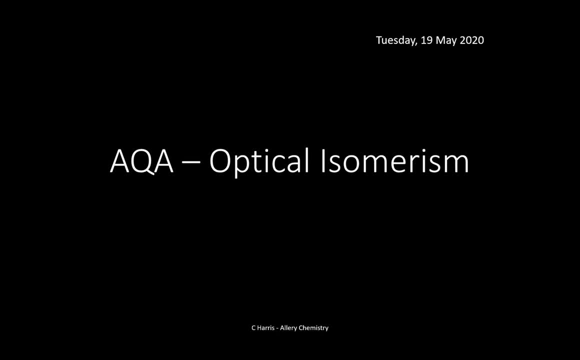 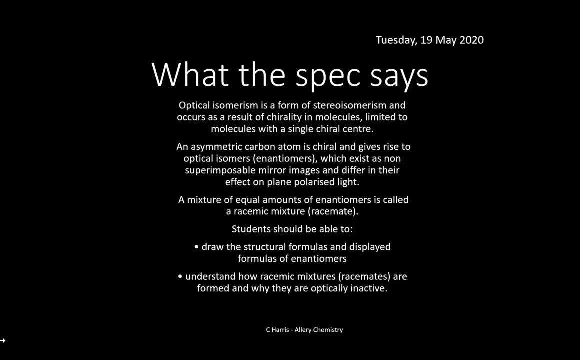 them from there. Like I say, they're great value for money. Okay, so, like I say, this is dedicated to AQA and so therefore it meets the specification points, as you can see on there. So we're mainly looking at optical isomerism, We're going to look at how we actually make optically active compounds. 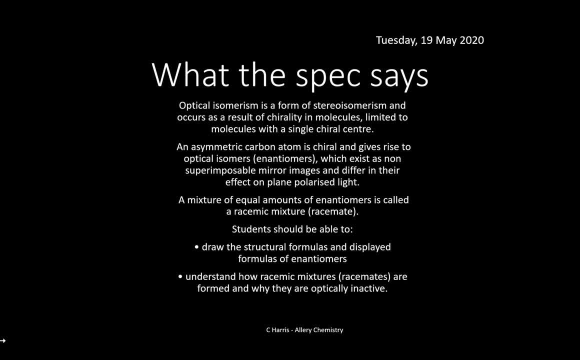 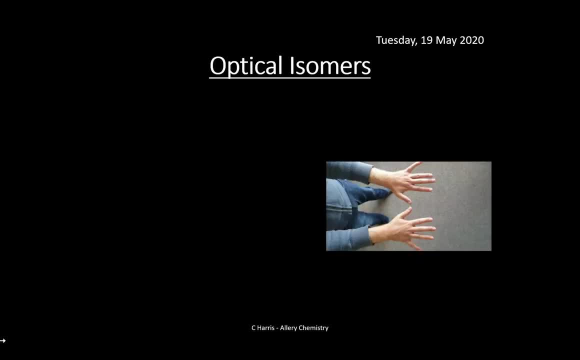 or substances contain the carbonyl group and we're going to look at racemates and enantemates. So some funny, strange words in this in this video here. Okay, so what we're going to do is going to look at optical isomers first. Okay, so you can see a picture of my hands there. I'll come onto that in. 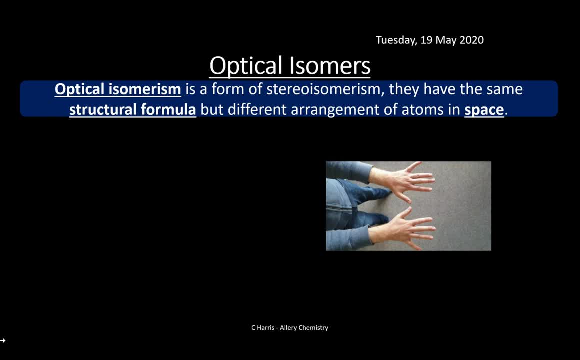 a minute. So optical isomerism is a form of stereo isomerism. So that means that optical isomers have the same structural formula but a different arrangement of atoms in space. Okay, so it's intriguing, I'll come onto this. You probably, if you've seen, if you've done optical isomers, you probably know. 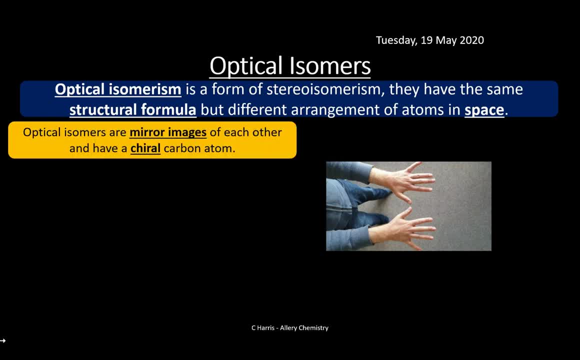 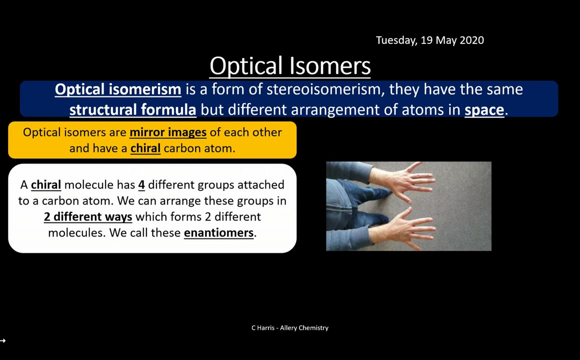 where I'm getting at with the hands. But yes, you'll see that in a moment. So optical isomers are mirror images of each other and they have a chiral carbon. Okay, so that's the carbon in the middle of a molecule. Okay, so what we mean when we say chiral is that the molecule, the atom. sorry, 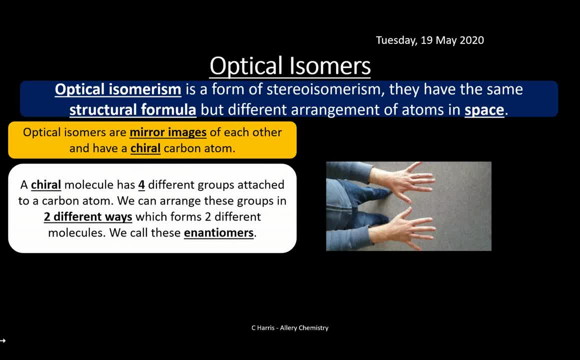 has four different groups attached to it and we can arrange these groups in two different ways and that forms two different molecules. We call these enantiomers. Okay, so that's very important. There's your first keyword. So basically, basically what that means is you've got a carbon atom and around that carbon atom you've got four. 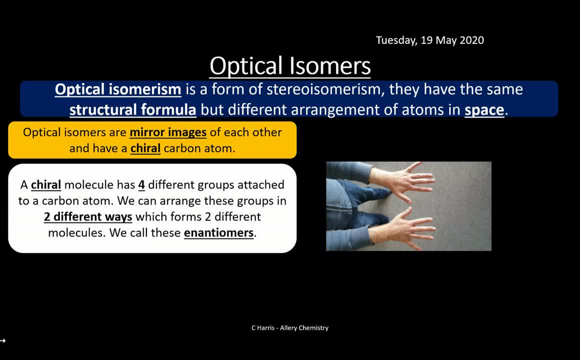 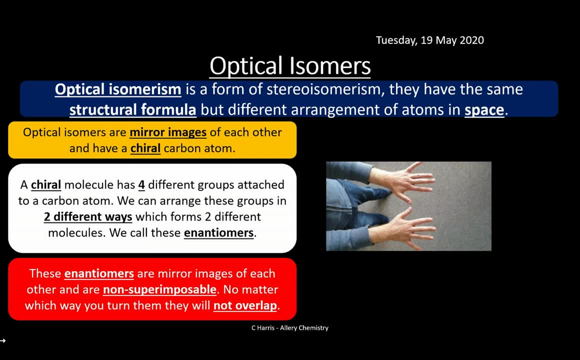 very different groups surrounding it, and that is a chiral molecule, And chiral molecules obviously have mirror images. You have two different versions of that molecule, So they're mirror images and we call them mirror images, enantiomers And basically what that means. an enantiomer is non-superposable. 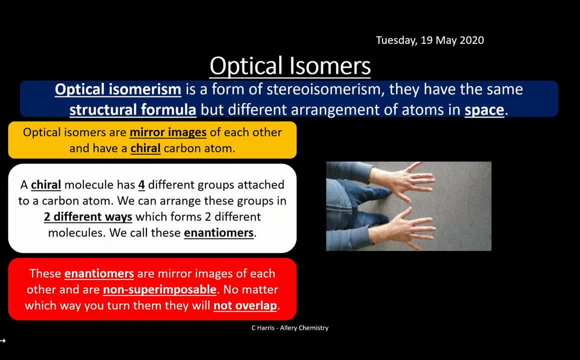 You can move it across, you know, over the top of another enantiomer, and it won't actually fully superimpose and it is a perfect mirror image as well. Okay, so this actually leads us on to what we mean in a kind of more tangible way, and that is hands. Hands have a chiral center and they're 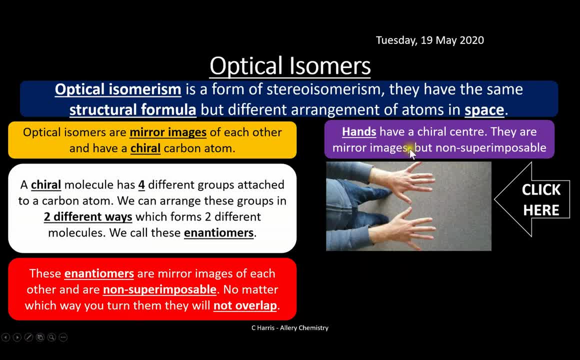 mirror images of each other, as you can see in the picture there. So you can see these are. this is a mirror image. You can see there's a if you put a mirror line down the middle. there there's a non-superimposable, as you're going to see here. So let's have a look. 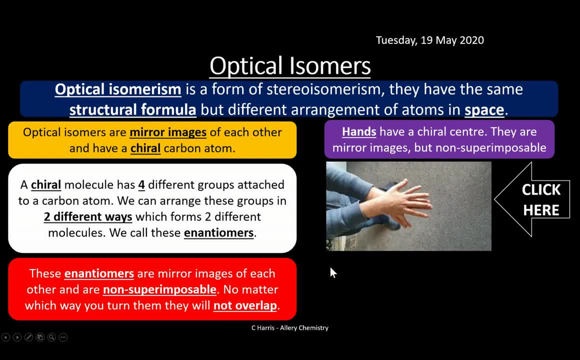 So there we are. Oh, it's breaking up a little bit So you can see there. anyway, I think you get the idea. when you see it, It will run smoothly, much more smoothly, when you, when you, if you, if you do have a hold of these, it's, it's because it's. I think it's working through this might. 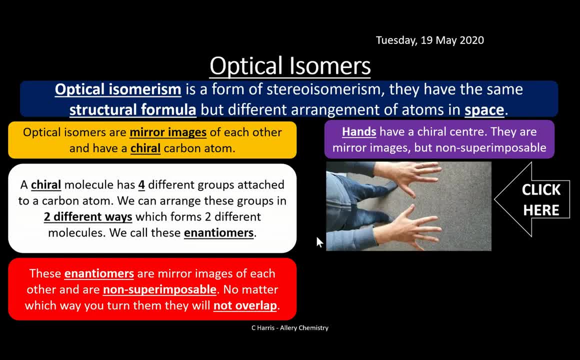 work smoother. there. There we are. that's better. Okay, there we are. Okay, so you can see that when we overlap the hands, I think it's because I'm running software alongside the hands, So I'm running software alongside this, So it's obviously slowing it down a little bit. So you can see when. 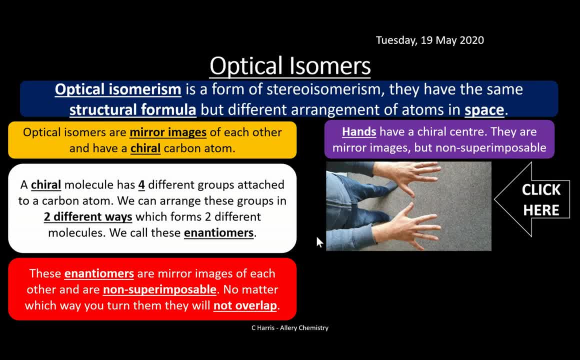 we put the hands above one and one another. they actually don't superimpose at all, But you can see the mirror images and we can apply the same principle to molecules. So let's look at it on a molecular level. So these two are enantiomers of each other and you can see, we've got the mirror. 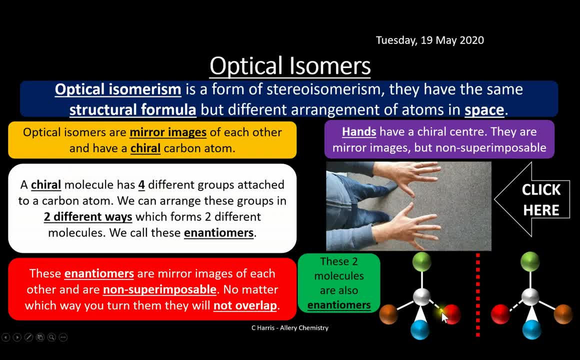 line down the middle there. So there's the mirror line there, So your mirror lines down there. you can see these are clearly mirror images of each other And if I take this one and put it over the top of that one, it doesn't matter how many times I orientate that, it isn't going to be the same. 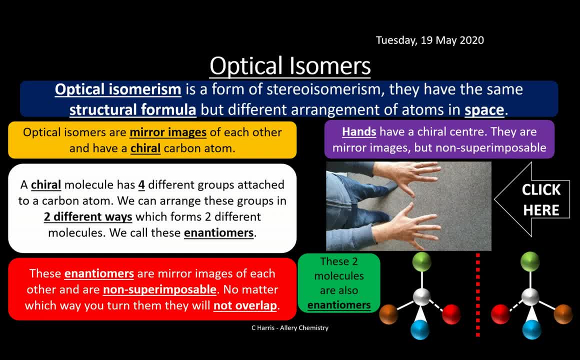 It's going to superimpose, It's not going to overlap. So that's what we mean. So we need to be able to find a chiral center, Okay. so that's quite, that's quite an obvious thing. So we know what a. 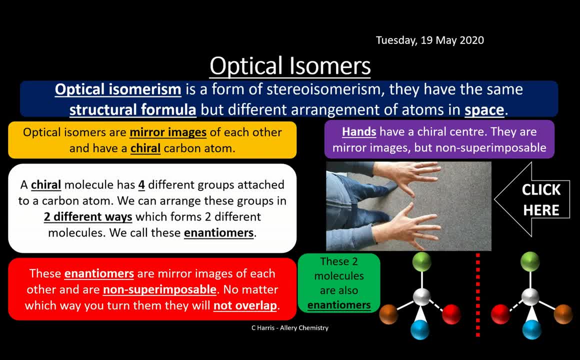 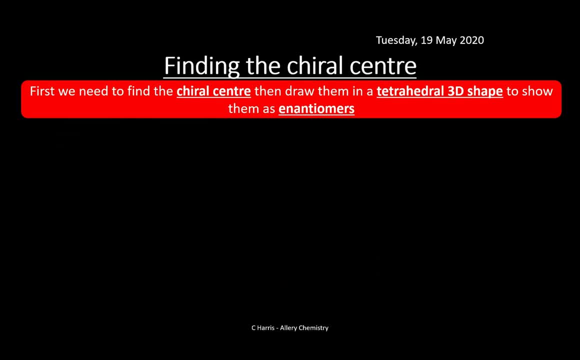 chiral center is. We know what we're looking for. We're looking for four different groups surrounding a carbon atom, So we need to be able to spot it. So let's have a look and see if we can find a chiral center. So first, what we need to do is, when we're finding a chiral center, we need to 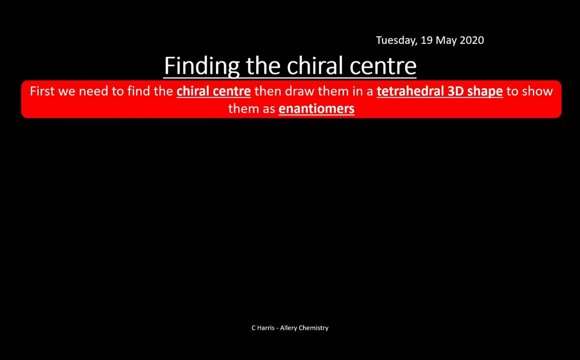 draw them in a tetrahedral 3d shape after we found the chiral center, And then we draw them as an atom, as we've seen there just on the previous slide. So first of all, here's our molecule here and we need to find our carbon atom. that is the chiral center We have. 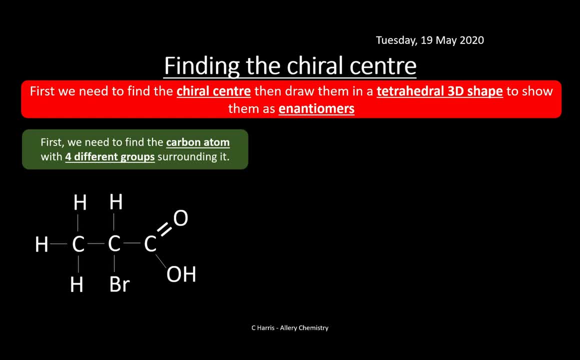 four different groups that we're looking for around it, So see if you can spot them. So one group is here, That's the blue circle there, Okay, so that's one. Second one is there, There, it is Okay. third one is there And the fourth one is obviously our carboxyl. 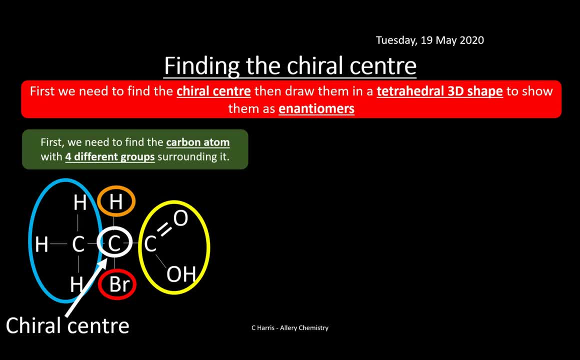 group. So you can see we've got a chiral center that's right in the middle there, because surrounding that carbon, you can see you've got four different groups surrounding the carbon in the middle. Okay, so then, what we need to do, once we've found our chiral center, we then need to draw it as a 3d. 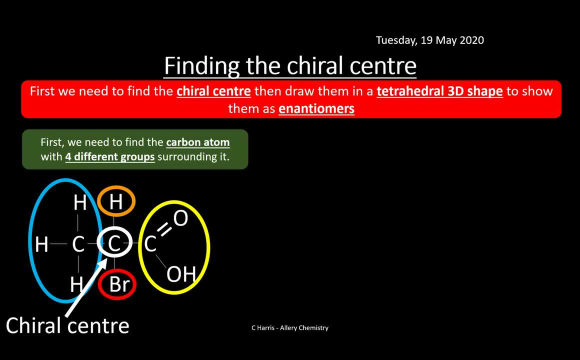 shape, So a tetrahedral shape, because we've got four groups coming from the carbon. So here it is, There we are. So remember you would have done this in year one, chemistry, when you drew 3d representations of molecules. So just as a. 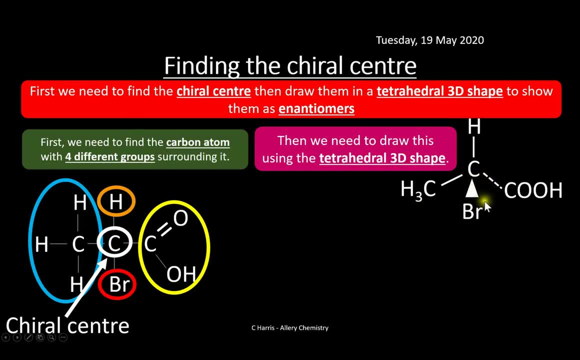 very, very quick reminder. you always have a wedge coming out, So this is an atom coming towards you and you have one that's going away, which is this one here. So this is your carboxyl group, with a line, a dotted line, showing a bond going away from you. And then these ones here, your 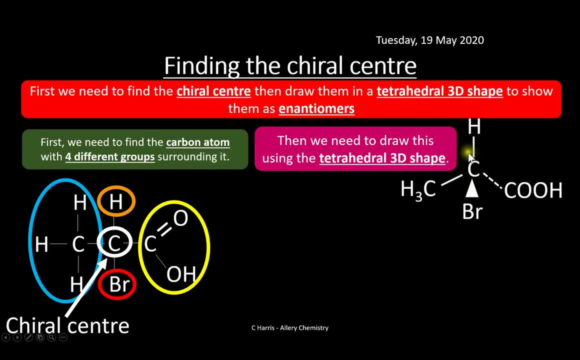 solid lines are in your plane of vision. So these are the ones that, if you were to look at it as a 3d model, they would be there, wouldn't be neither coming towards you or going away. So they're in your plane of vision. So just a reminder of how we draw them: 3d, 3d molecules. So once we've 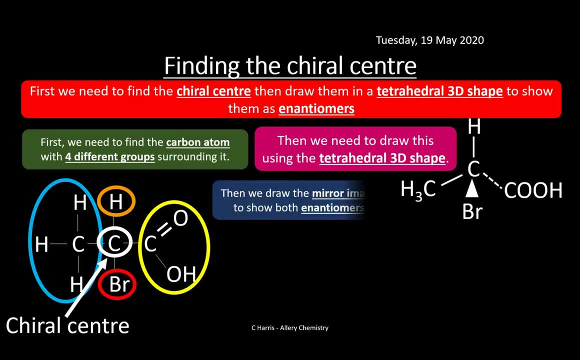 drawn our 3d shape. we then need to represent them as enantiomers. So you can see, we need to draw a mirror line, mirror image to show them, to show the two enantiomers. So here it is, here, OK, So you. 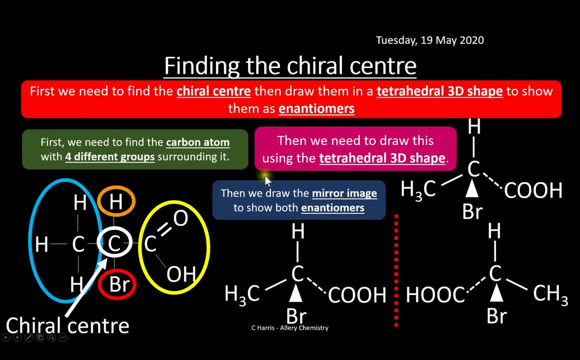 can see that this molecule is definitely 3d shape and you can see that it is definitely an enantiomer of each other, because the mirror line goes down here and this is a mirror image of this And if you put them over each other they're non superimposable. So the main criteria is looking 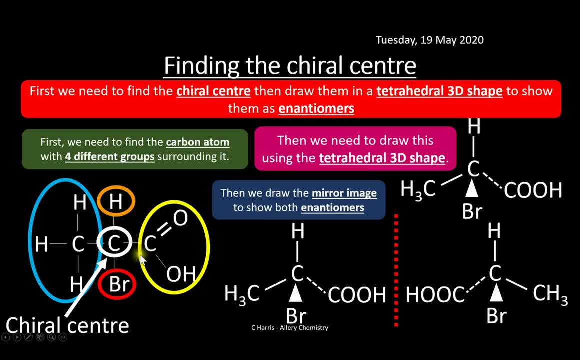 for these four different groups. anything, any four different groups around the carbon is actually chiral. And if it's chiral, it will have two enantiomers, 11 mirror image of each other. OK, So how do you actually spot these? because if you, if you look at these, it's really difficult. 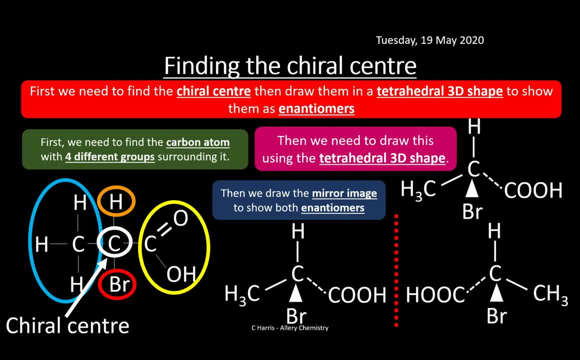 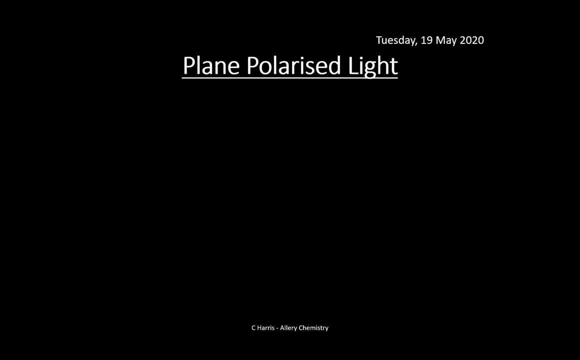 They've got the same molecular formula, the same functional groups and you'd be thinking, well, how on earth do you actually spot these things? How do you detect them? Well, what we use is we use something called plane polarized light, OK, And so if we have a chiral center, we say that 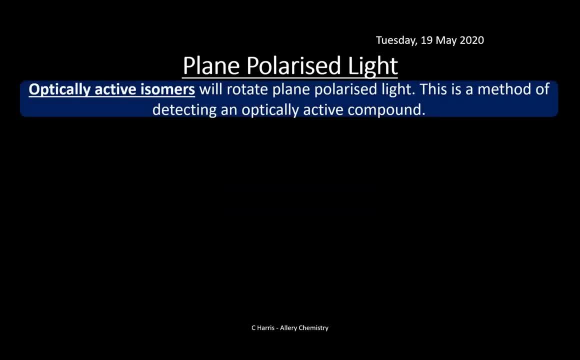 molecules of the chiral center are optically active. OK, So what that means is that they will. they will rotate plane, polarized light And effectively, if we have a molecule in there that is chiral and rotates plane and it is chiral, then it is optically active. Then if we shine light, 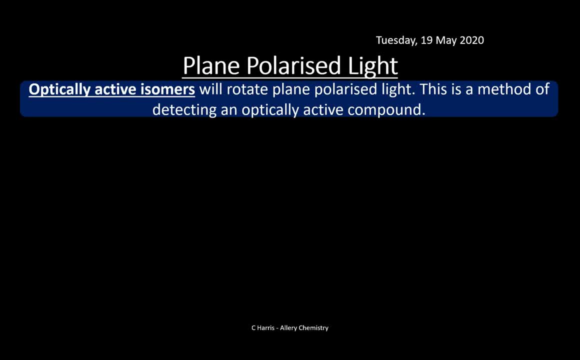 through it plane polarized light, then it will rotate it. Now the next thing is: well, what is plane polarized light? Well, I've got this really handy diagram to show you. So you've got normal light. So this is standard white light that comes through the windows. come through the window, right? 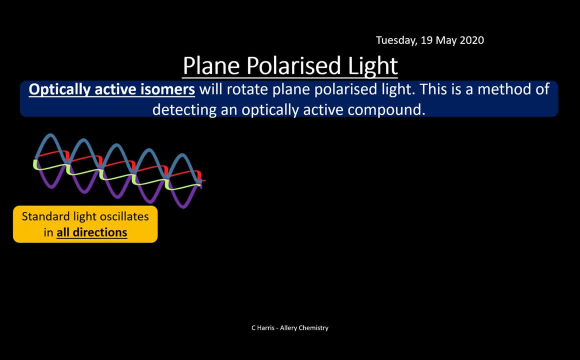 now that I can see It has low. it has low, A variety of different frequencies in there, And if we just pick one frequency then they're oscillating in many different directions. OK, So that's standard light. So that is no good We need. 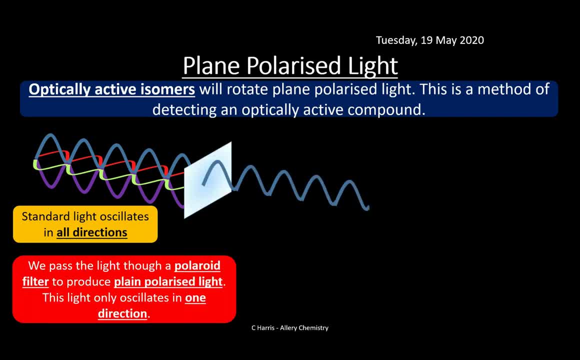 to polarize this light. So what we do is we pass it through a polaroid filter, and a polaroid filter blocks most of the directions or most of the orientations of the light and only allows one orientation to go through. So you can see here, this is now plane polarized light. 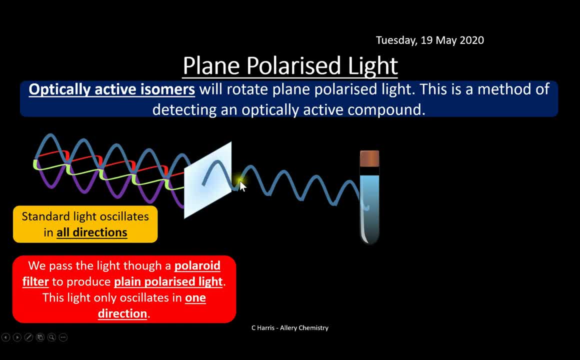 So we have blocked all of the other orientations apart from this blue one which has come through the filter and it's only oscillating in one direction. So then what we do is if we've got our optically active compound in here. So let's say there isn't a chiral center in this, in this. 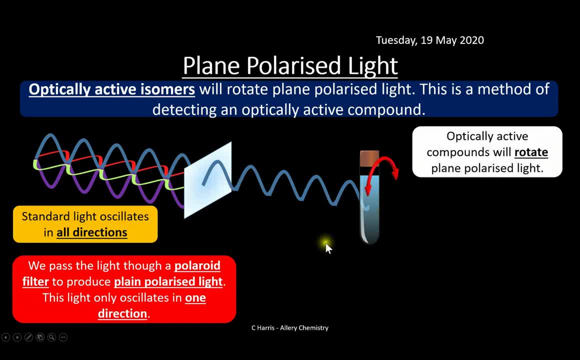 solution here, then what will happen to this plane? polarized light is it will rotate, and it will rotate left or right. So very straightforward. However, what we've got to look at is: remember we said there was two enantiomers in our, in our room for 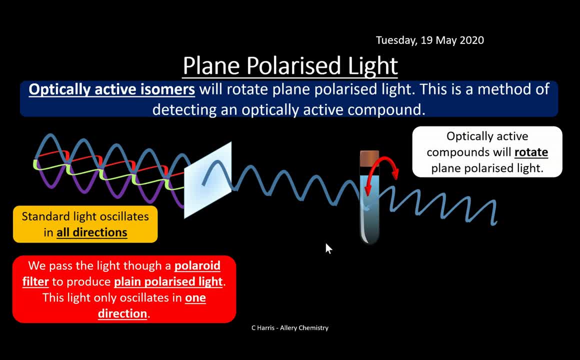 every optically active compound, it will always have two enantiomers. Now you might have more of one enantiomer than the other, which is fine. It means you'll get an overall oscillation, but basically how you distinguish between each enantiomer is one of the enantiomers will rotate. 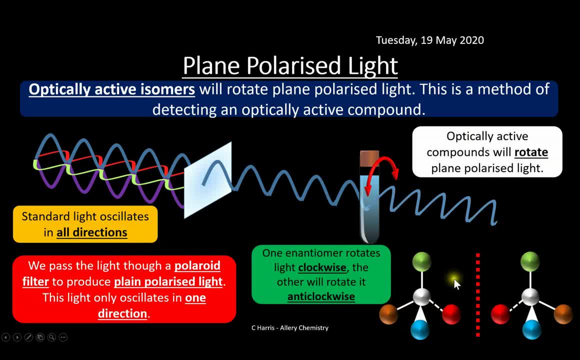 it. Here's your two enantiomers. So one enantiomer will rotate it clockwise and the other enantiomer will rotate it anti-clockwise, but they'll both rotate it by the same level of degrees. So, for example, if this one is rotating by five degrees clockwise, then the other enantiomer will rotate. 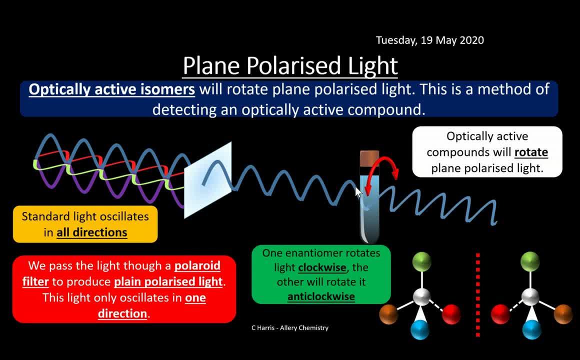 five degrees anti-clockwise, So the degree of orientation is the same, it's just each enantiomer will rotate the light in opposite directions. So that's very, very important and it allows us to identify. obviously, if there's a majority of one enantiomer over another, then you'll get an overall. 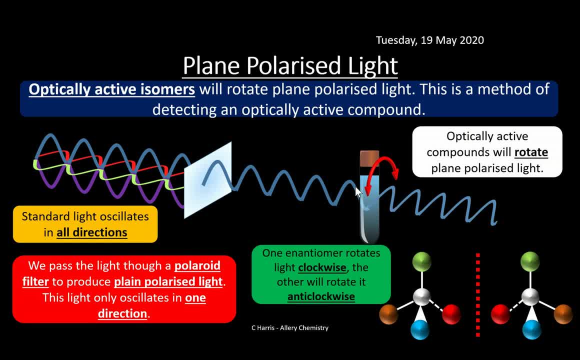 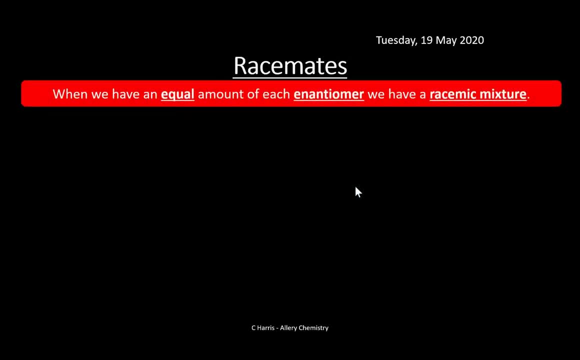 rotation of light. Now the problem comes when, actually, you've got an equal amount, and when we've got an equal amount of each of these enantiomers, we get something called a racemate. So a racemate is just an equal amount of each enantiomer. 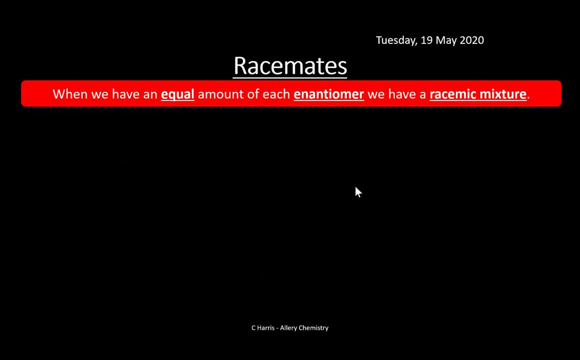 And we have what we call a racemic mixture. Okay, so that's where we have a 50: 50 mix of each enantiomer. Now, racemates do not rotate, plane polarized light and this is because both enantiomers rotate. obviously you've got equal amount of each enantiomer and they're rotating in opposite. 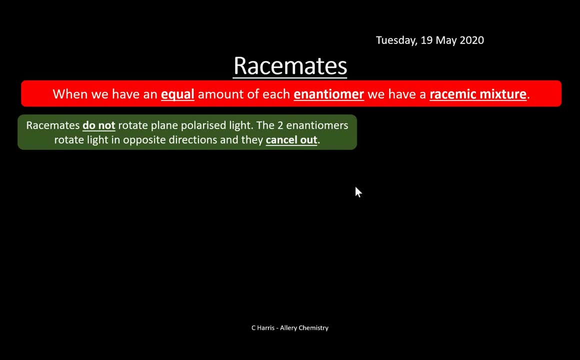 directions. So the net effect is zero. there's no rotation. Now you've got to be really careful with that, because just because you shine light through a plane, polar, a sample, and it doesn't rotate, it doesn't mean that you don't have optically active compounds in there. Be really, really careful. 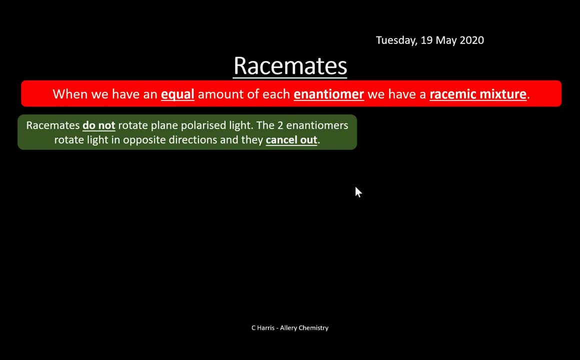 with that in the exam because they will say, oh look, it doesn't rotate plane polarized light and automatically you might think, oh well, it doesn't have a chiral center, so I'll just get rid of that. open your mind and look at something else. It might have a chiral center, it's just you might. 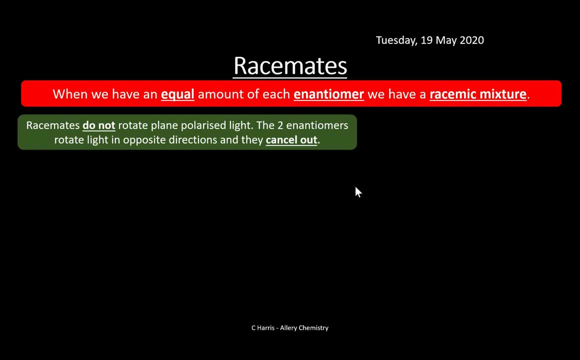 have a 50: 50 mix of each enantiomer and therefore you form an erasmus. So you can see, a racemic mixture of a chiral product is often made by reacting achiral substances together. Okay, so if we have something, basically two substances which don't have a chiral center, 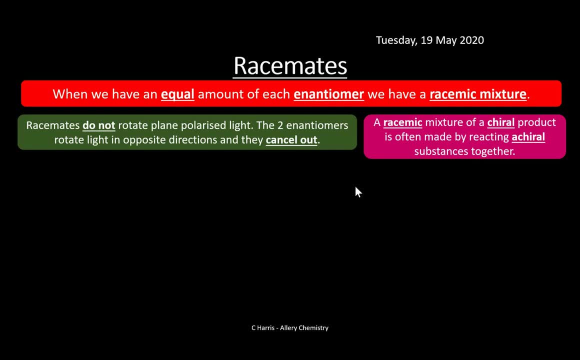 normally, when we add them two together, we can form a chiral center. Okay, so when the molecules, when the molecules react, there's even a chance of forming a forming each enantiomer as well, so we can actually form. you know some, one enantiomer and another enantiomer, Some reactions, you only 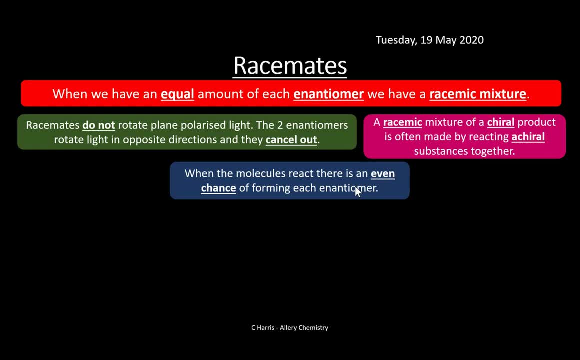 get one, we majority, we get one type of enantiomer. So let's have a look at an example So you can see, here we've got our alkane, which is here. this is alkane, and we're going to react it with a halogen, or halidine, should I say, which is Br minus, So that will form this type of compound. 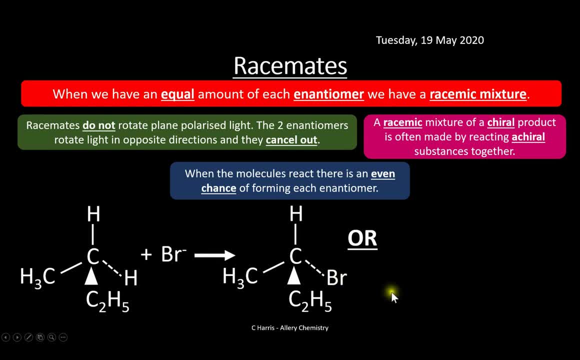 here and you can see this. carbon's got four different groups surrounding it, so that's chiral or it can form. it can form this where actually the halogen is actually at the top there. So you can see that neither of these are chiral, because we've got two hydrogens there, so they're the same. 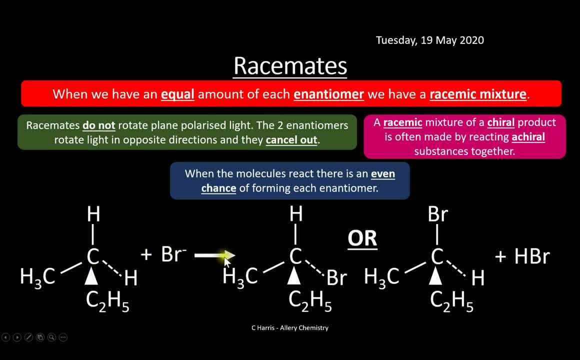 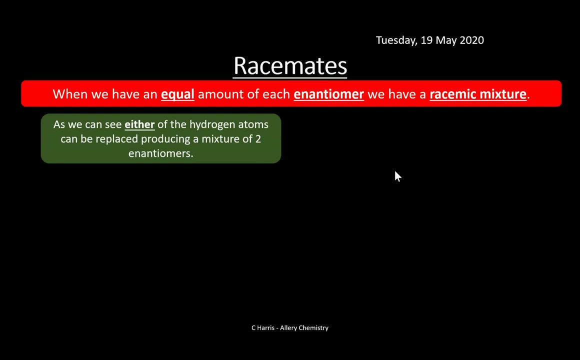 four different groups, but actually, by reacting it with two non-achirals, we can actually form chiral compounds, as you can see here. plus we can form a hydrogen bromide. Okay, so we can see that as, like I say, either of the hydrogen atoms can be replaced and what we do is we produce a mixture of. 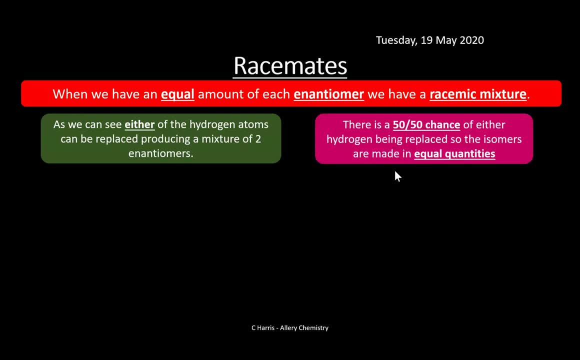 two enantiomers, as you can see on there, and obviously there's a 50-50 chance of either hydrogen being replaced. so the answer: so the isomers are made in equal quantities. It doesn't. it's not always the case that you always get 50-50 mix, and sometimes you can get the majority of one. 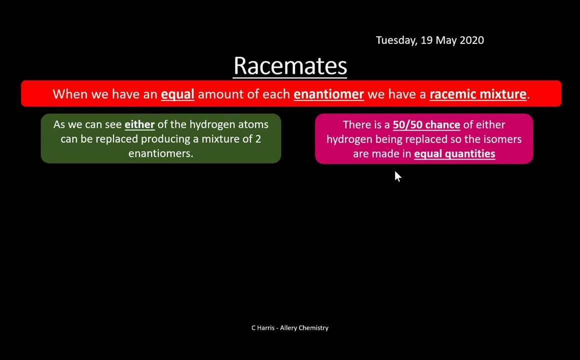 enantiomer and very, very little of the other enantiomers, so it can be heavily weighted towards one side. So sometimes you just get. you know you only produce one enantiomer depending on the reaction. you know, but there's always with enantiomers there's always. you know it's a. 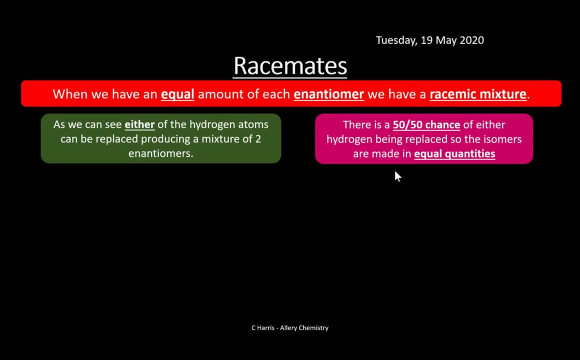 mirror image. it always has a mirror image. it doesn't mean practically that you are going to produce that. Okay, so you can see. here's the diagram here. so these are the two molecules that we've just seen before and you can see they're clearly mirror images of each other. you've got. 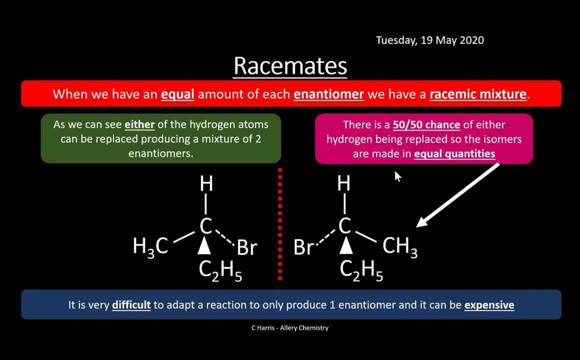 the mirror line down the middle there, and obviously both of them are enantiomers. So it's really difficult to adapt a reaction to only produce one enantiomer. it can be expensive and then you might be thinking also: what, why do you only need one enantiomer? what's the point? why would you? 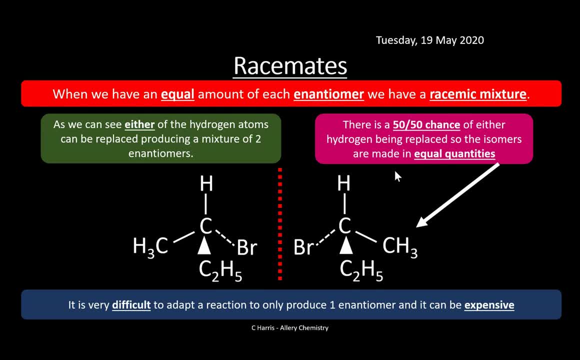 just just let it produce both. Well, you might have heard of a case years ago called thalidomide where people would make for morning sickness. so for people who were pregnant and suffering morning sickness then they could take thalidomide. Now one of the enantiomers of that drug was 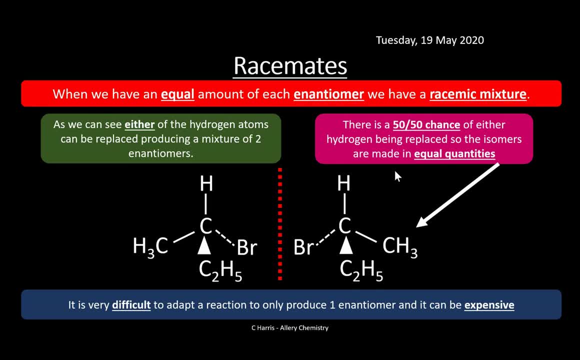 successful at doing that and the other enantiomer actually was dangerous and caused deformities in children and you get, you know children and obviously this is many years ago. you know they'll be considerably older. you know considerably older now because this, this happened back in the 60s. but you know these people were born and were 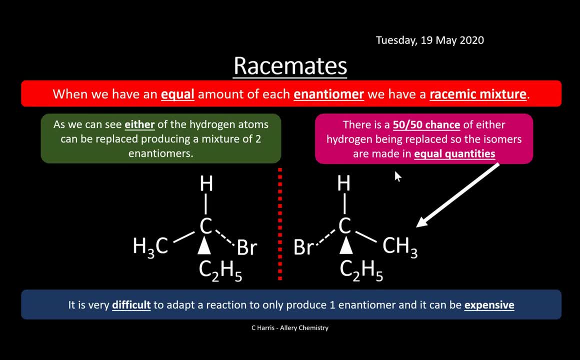 born with deformities and maybe missing limbs or, you know, stunted limbs etc. so it is really important, especially in pharmaceuticals, that if we are producing the drug, that you know, if we are keeping both enantiomers in there, we've got to make sure that obviously the useful one is doing. 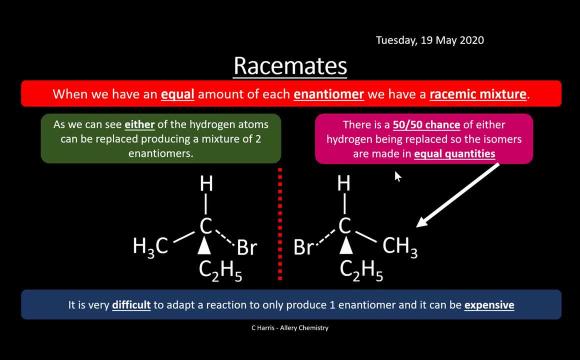 what it needs to do, but you know the one that isn't required. does that have any side effects? and if it does, we've really got to try and remove that enantiomer, You know. if it isn't, you know there's loads of, it's very common to have, you know. 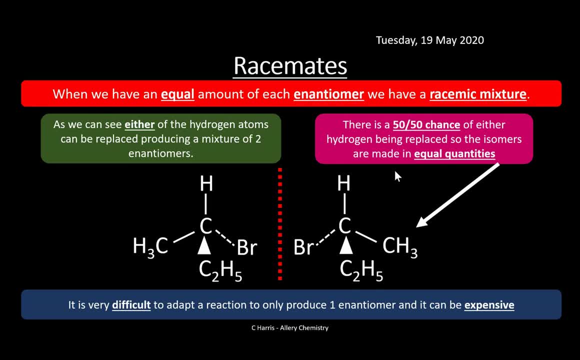 it doesn't take a lot to have optically active compounds. you might find that the other one just doesn't do anything, you know. so one of them might actually cure the disease it's trying to cure or relieve pain etc. and the other one might do absolutely nothing. there has no side effects, so 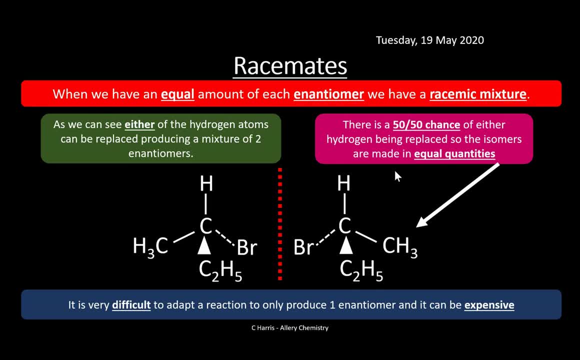 there's no point in removing it if it doesn't have any any significant impact. so so it is cost. it's all down to cost. you know, it's all one thing, it's all well and good producing a drug, but if it costs hundreds and thousands of pounds to buy, you know, then you might think that's. 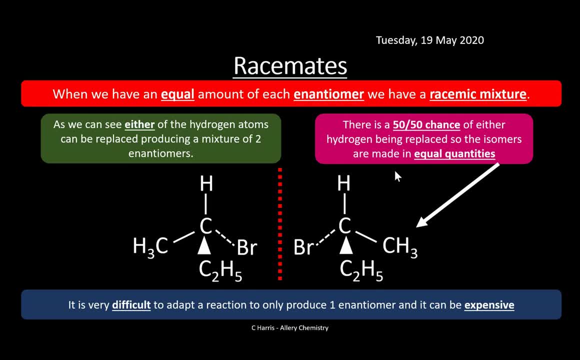 well, you know, is it is it, you know, is it, is it viable? you know. so you know drugs cost a lot of money and and health services, particularly obviously if you listen outside of the UK, but particularly in the UK, you've got the NHS, which is the the buyer of these drugs, and they're made 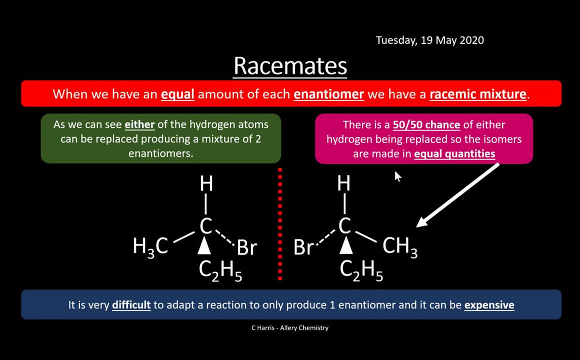 by private companies and so you know there's a cost to every drug and they've got to try and work out. is there a cost benefit analysis? and not all drugs are. you know are economically. obviously every drug is viable. you know if it's going to help somebody's life or save their life. but you know there's a cost to everything and if there isn't any money to buy it it can be quite difficult maybe to justify if it's only going to maybe cure one or two people's lives and you know if the drug is more widely needed, then obviously you know there's a there's a cost, there's a cost. 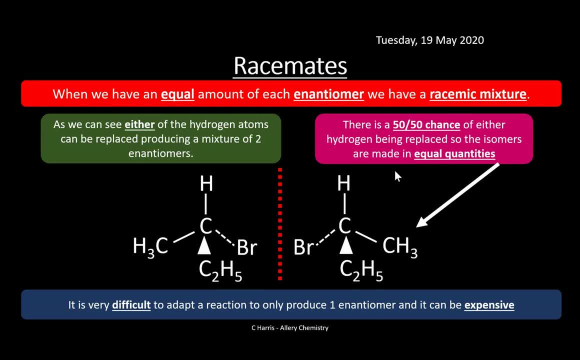 associated with that. so basically, we've gone off a bit topic here, but you've got, you know, you've got to weigh these things up. there's a cost and is it worth it to make the drug? is there a you know? is there is there a benefit of of doing the drug or is there another way of making it? 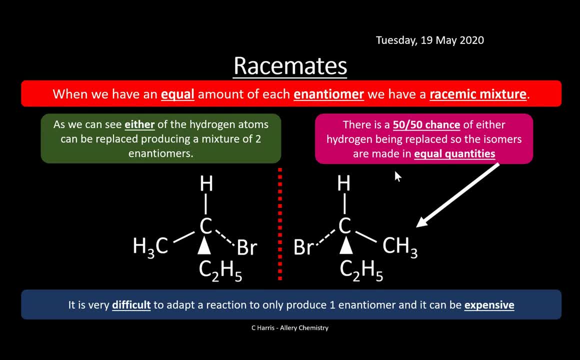 so this is why drug development takes years to come up with, because we've got to look at tests, you've got to trial it, you're going to make sure it works and racemates form a massive part in drug development. um, you know, enantiomers- enantiomers in that in that case, and we've got to make sure. 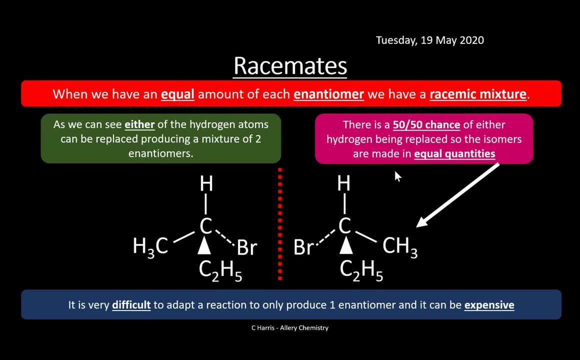 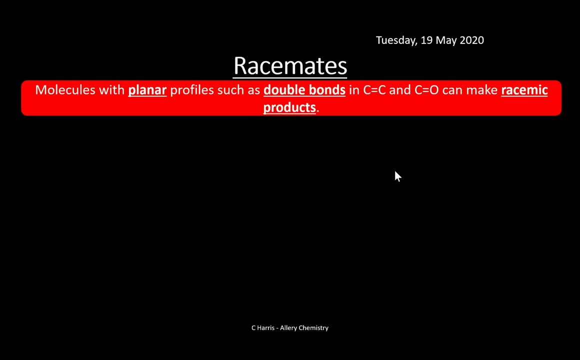 that you know? um is the enantiomer. is it worth taking it out of the drug, so? so that's what we've got to look at here. okay, so um, molecules with planar profiles, such as double bonds and cc double bonds and c double bondo, can make racemic. 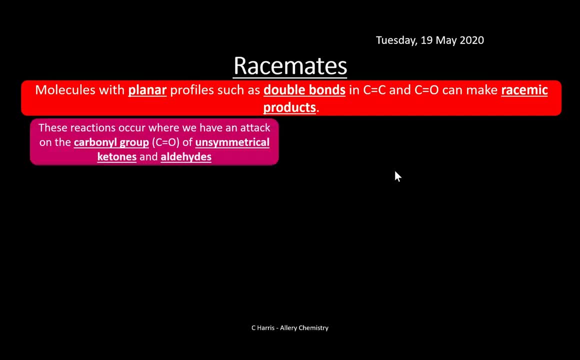 products. okay, so this is quite important because we're going to look at a mechanism here. so these reactions occur when we have an attack on the carbonyl groups, that c double bondo group, c- double bondo group, um of an unsymmetrical ketones or aldehydes. okay, so you would have. 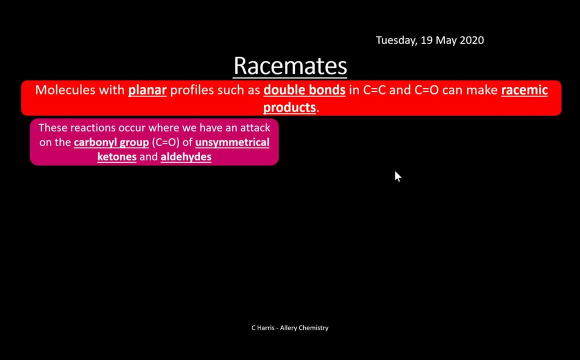 seen this um before um, you might have seen aldehydes and ketones before um, in particular making carboxylic acids, for example. now we're going to look at an example where propanol reacts with acidified potassium saline, so kcn in this particular example. so we have, as you can see here, unsymmetrical, an unsymmetrical. 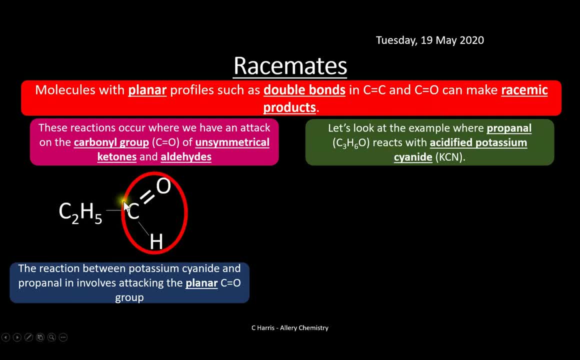 ketone. okay, so we've got, uh, this is an aldehyde, sorry, an unsymmetrical aldehyde. so you can see, here, this bit is um, is is planar, okay, so this is the planar bit. this bit's flat, this bit has um bits sticking out everywhere. obviously i've drawn it in this way, um, you know, because that's the 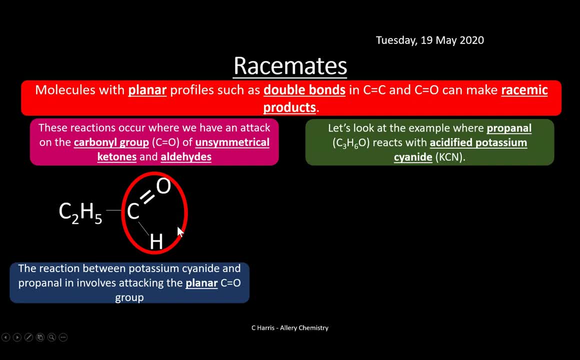 standard way of drawing it. but this bit is the planar bit, this bit's flat, okay. so if we built it onto one side we can actually see it, we can actually see it drawn out there. so as part of the um, uh, so as the c double bondo, that should say part, not pattern. i don't know who that is um. so as, 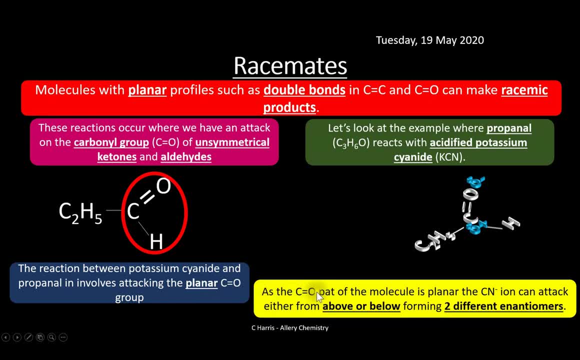 the. i'll get that changed, of course. um, so as the carbonyl group, the c double bondo part of the molecule, is planar, this bit, the cn- minor sign that we're going to react this onto- can attack from either the above or it can attack from below, and this forms two different enantiomers. so let's have 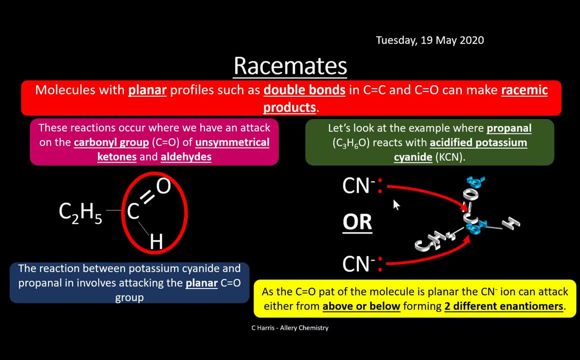 you see the cn minus attacking from the top or from the bottom. so you can see here that these are um nucleophiles and they have a lone pair of electrons. so they're nucleophiles and they're attacking a delta positive carbon in the middle and you can see it's got an equal chance of it. 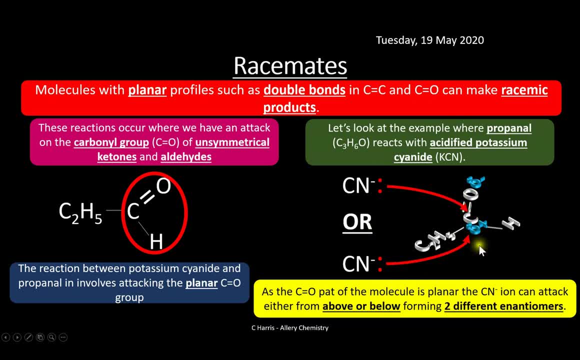 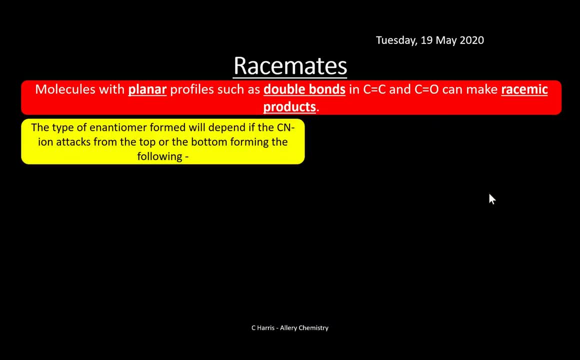 reacting at the top or reacting at the bottom. um, you know, there's there's, no, there's no other groups there that would hinder it one way or the other. so the type of enantiomer formed will attack from the bottom. so you can see here, if it attacks from the top of the bottom, we get two. 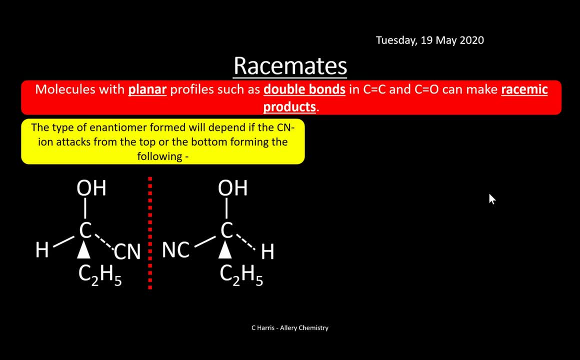 different enantiomers. so we get both enantiomers here, as you can see, and they're mirror images. so we know there's a chiral center there, chiral carbon. so due to that planar nature of that carbonyl group there's an even chance of the nucleophile attacking from the top and from the 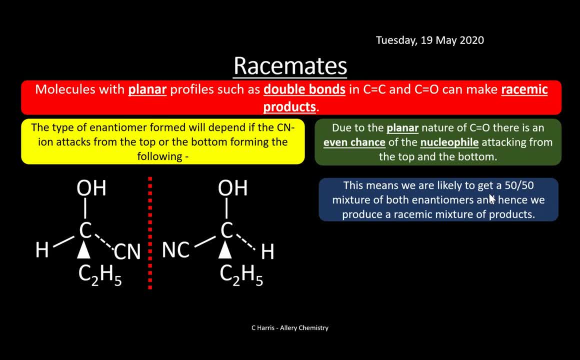 bottom. so there's no preference, like i say. so what this means, um, is that we're likely to produce, obviously, a racemic mixture, and so it's a racemate, because we're getting 50: 50 mix, and we're getting 50: 50 mix of each enantiomer, and so, as with all racemic mixtures, they don't rotate plain. 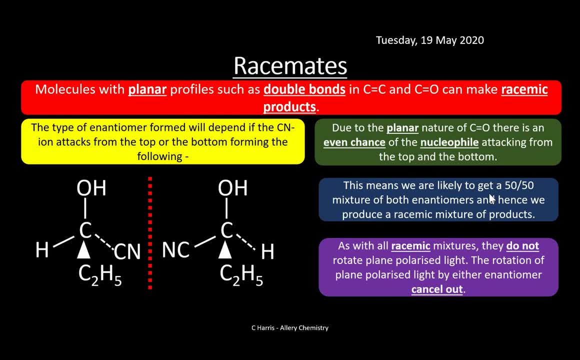 polarized light because the rotation cancels out on each of them. um so um. that's really really important. that's that you, that you're aware of that. i can't stress that enough. just because it says it doesn't rotate plain polarized light doesn't mean it's not, doesn't have a chiral. 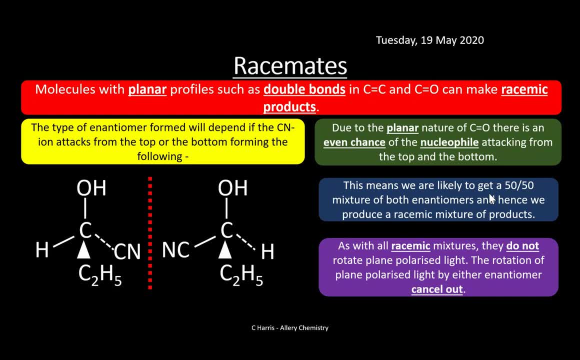 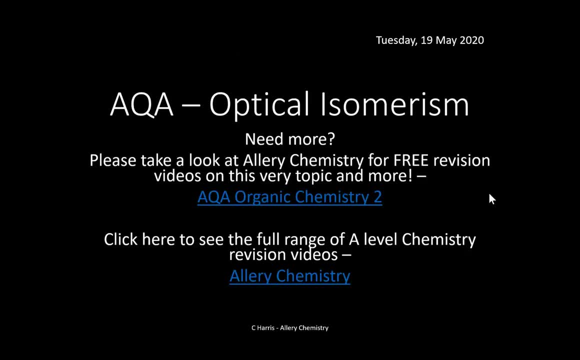 center, as you can see here. it can have a chiral center, it just might be a racemate. so just have that in the back of your mind and just make sure you, you know you score that off. okay, and that is it. so that's it on optical isomerism. um, so, quite a short topic, relatively speaking, um, but you do. 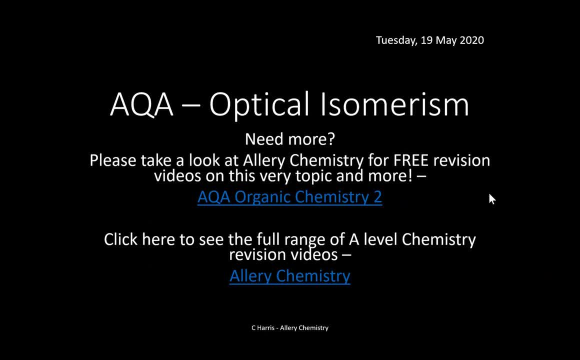 need to know about, obviously, a lot of keywords in that one, like racemate, uh, enantiomers, um. you know your 50- 50 mixes, for example. so you know there's a lot of uh, you know terminology that you need to be able to express in the exam and, like i say, there's a full range of videos, though. 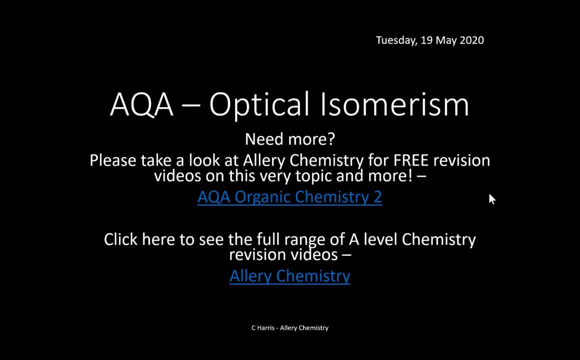 for aqa um for year one and year two chemistry um. go and have a look there, as well as for other exam boards as well. um that i've done. go and have a look. it's on alloy chemistry youtube channel um the full range of whiteboard tutorials and exam pipe exam past paper questions as well. so 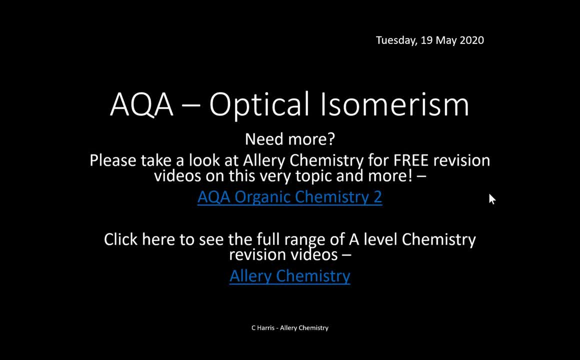 there's loads of stuff on there and it's constantly changing, all for free. all i ask is you please hit the subscribe button. that'll be fantastic. um, and also, these are available to purchase as well, but just click on the link in the description box. great value for money and great revision material.